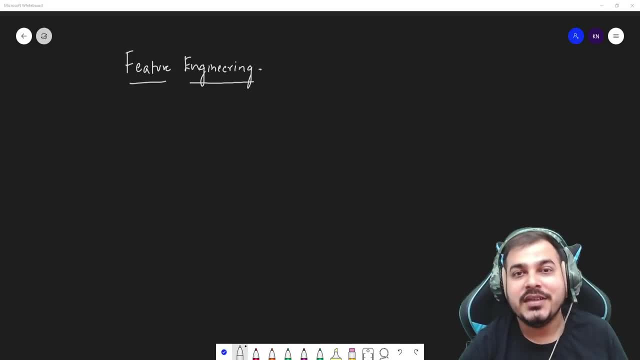 Hello, all my name is Krishnayak and welcome to my YouTube channel. So, guys, today, in this particular video, we are going to discuss what all steps we actually perform, in what kind of order, to complete the feature engineering process. Now, in a data science project, guys, if I just consider feature engineering, it takes somewhere around 30% of the entire project time, right, 30%? So it is very, very huge. you know, and there are many, many people who have asked me questions. 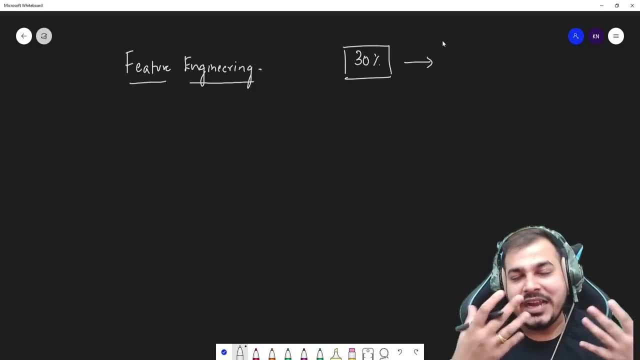 Like Krish, what is the exact order? See, after I get the data, the raw data, what should I first do? You know, and if you remember, in the lifecycle of a data science project, the first module that actually comes is feature engineering. And then, after that, feature selection, then you have model creation, then you have model deployment, then you have hyperparameter tuning. Before model deployment you have hyperparameter tuning, Then you also have incremental learning, And there are many more steps as such, But the most 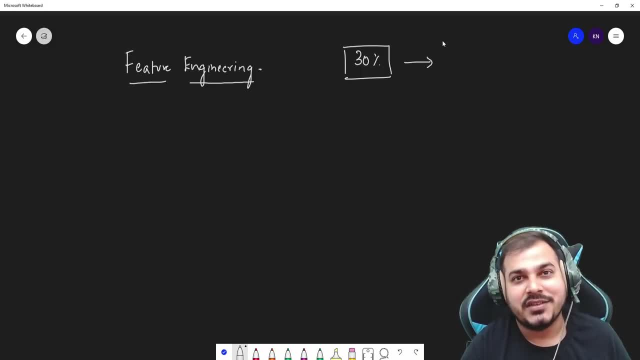 important. the crux, the backbone of the entire data science project is feature engineering, because you will be cleaning the data. you'll be doing a lot of steps, So let me talk about every step that you may be performing in feature engineering, step by step. Okay, So the first step that I want to discuss about is- I'm just going to write it down- The step one is basically EDA. Now, EDA is nothing but exploratory data analysis. 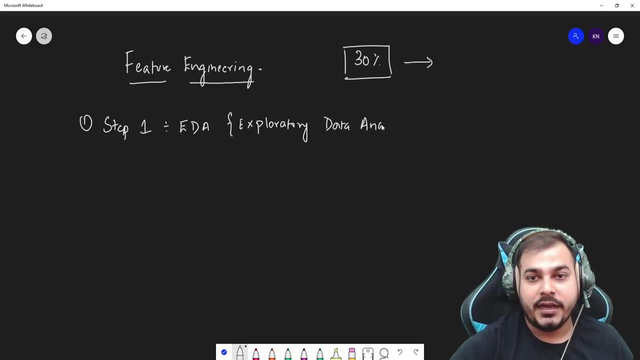 Exploratory data analysis. Now, this is a very, very important thing And remember guys, in my YouTube channel I have created dedicated playlist on feature engineering, on EDA, everything, So I'll also be giving those entire link at the last, Okay. So first step, step one is basically EDA, that is, exploratory data analysis. Now you may be thinking: okay, fine, exploratory data analysis. 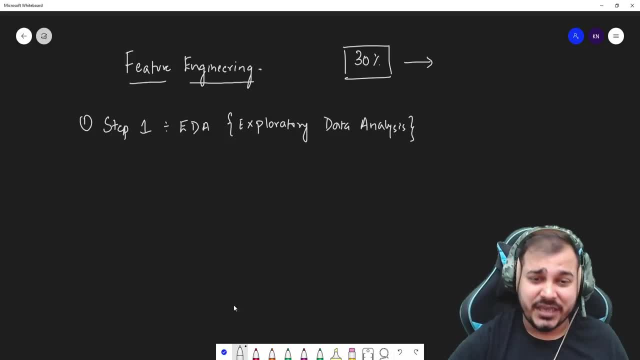 This wouldn't only be about exercise analysis in the EDA. you need to ask: you know balancing, and is it only about data analysis? No, there are many, many steps that we actually perform in this, So let me write it down one by little bit. 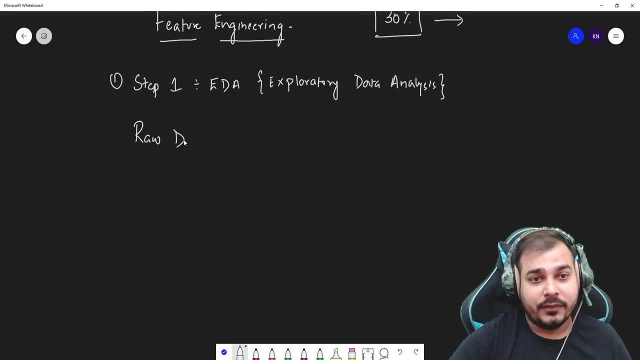 in EDA as soon as we get the raw data. okay, as soon as we get the raw data, because the entire feature engineering is actually done on the raw data itself. So, as soon as we get the raw data, what do we do? we start doing the analysis. now, What kind of analysis area do? 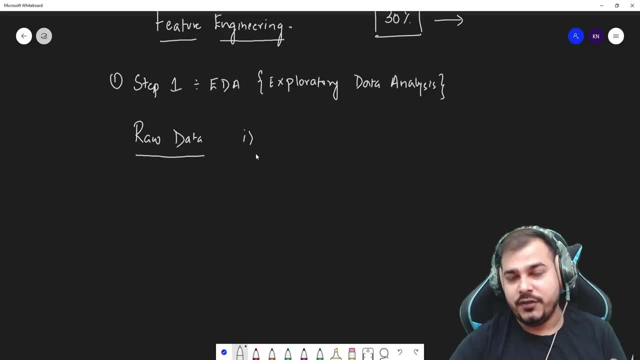 First of all give you one example, first of all, what i actually follow. as soon as i get the data, i basically see that how many numerical features may be there? okay, how many numerical features may be there, all right. then i may go up with how many categorical or discrete categorical features. 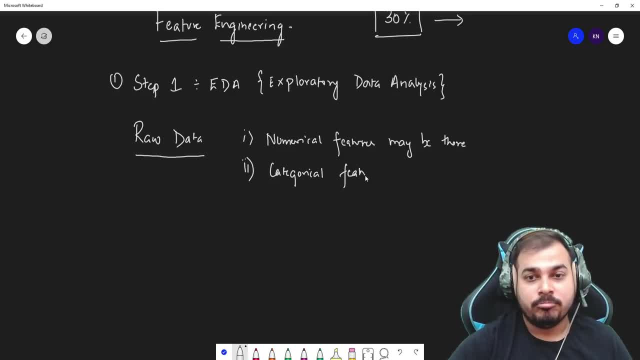 may be there. categorical features, i may. i may try to see this. numerical features: i'll try to just define or draw different different diagrams like histogram, right, like pdf function, right, and obviously you know all these things. you can use libraries like seaborn, right? i hope everybody is familiar with seaborn. we use seaborn, you know. you can also use matplotlib to see all this kind. 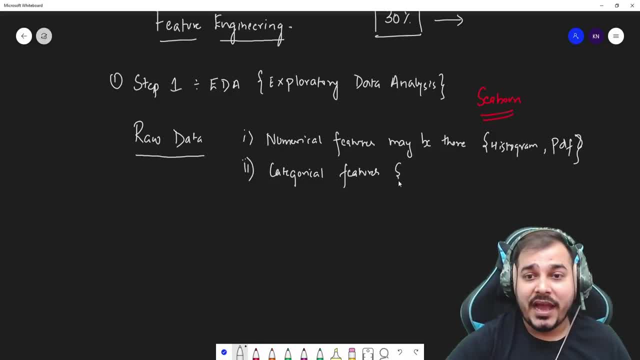 of diagrams right and then in the category features you'll try to analyze the category features, like: how many category features may be there? you know in those features how many categories may be there. is there multiple categories? see, all this observation is actually necessary. you know, all this observation is basically very 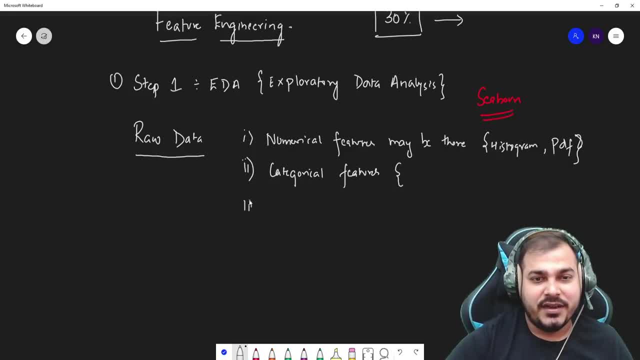 very much necessary. okay, now, coming to the third step that i will definitely follow. i'll just try to see whether there is any missing values. i will just try to clearly draw, clearly draw visual. or i'll just say: i'll try to visualize all these graphs. visualize all these graphs. 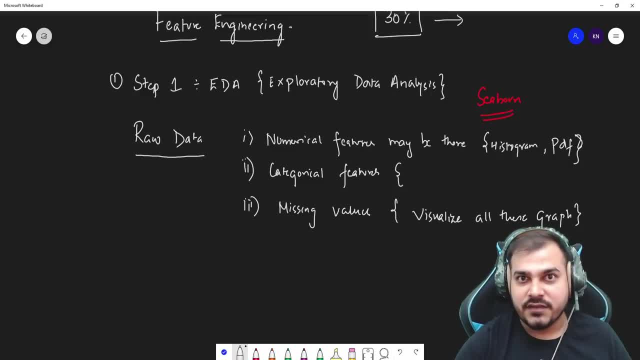 you know, with the help of missing values. also, if there is any missing values, i'll try to see. you know, probably, uh, i may go with my fourth step. i'll try to see whether there are outliers. and how do you draw an outlier? simple box plot, right box plot. i'll go with box plot, i'll try. 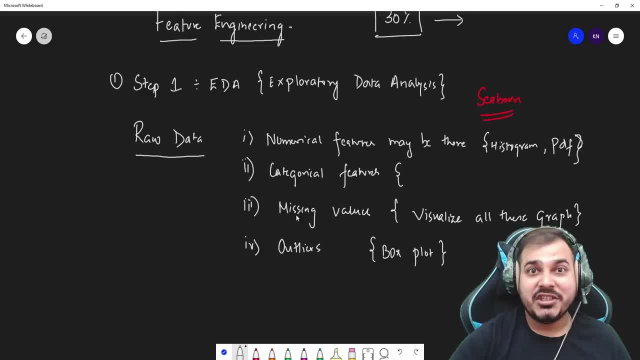 to see whether there is any outliers. now. these observations are very much necessary because whatever diagrams you are actually drawing, this all needs to be sent to your manager, to your, because that is what you have done in the eda right. and this is just a the first step in the 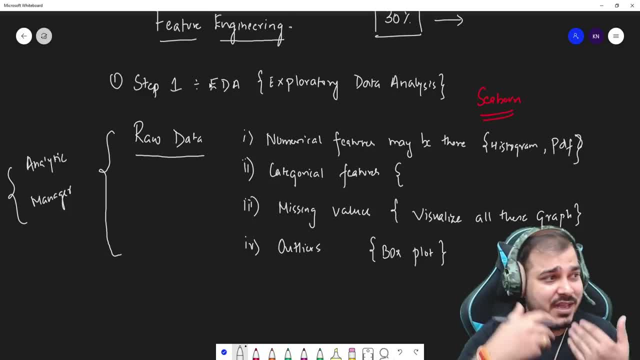 entire feature engineering and, trust me, there are many more steps which i will be telling you in just a while. right outliers missing values, category features, numerical features, and you know there are various. there are three to four different types of uh handling missing values. missing values will be because of different, different reasons and based on that, you have to 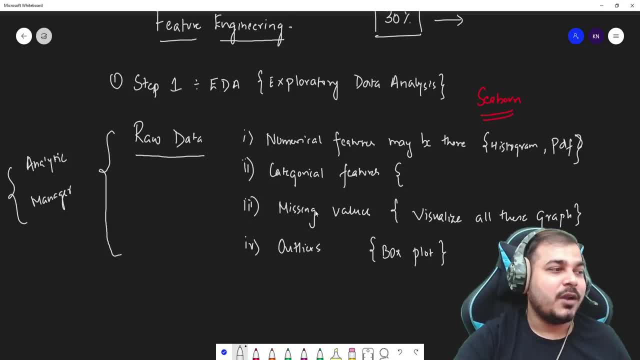 act accordingly. right so you have outliers. probably you know you'll try to see, uh, whether the raw data needs cleaning also or not cleaning or not. right so this, this is also a very important step. the raw data may have many information in just one feature and out of that. if you want, if you require all those information or 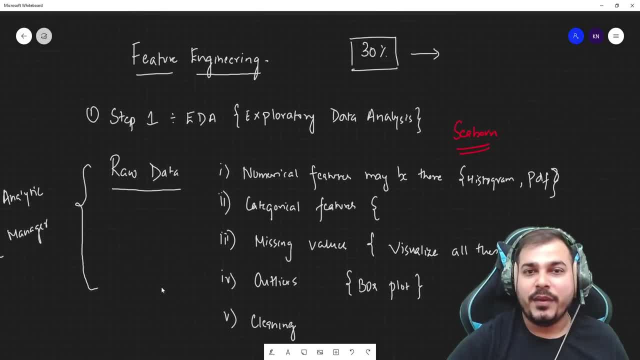 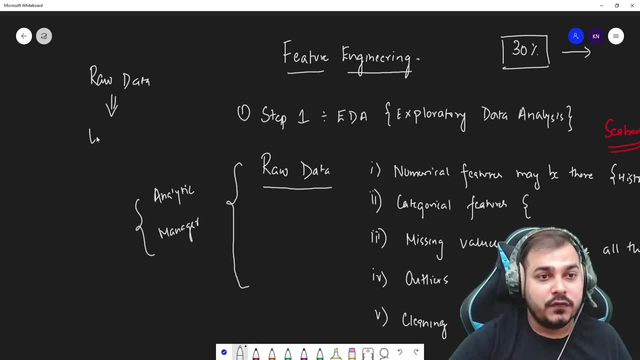 not right. but again, understand the main step over here, what we are trying to do. we are trying to convert the raw data into useful data. useful data so that our ML algorithms will be able to ingest them properly, ingest them for giving amazing predictions, right? so in the EDA part we 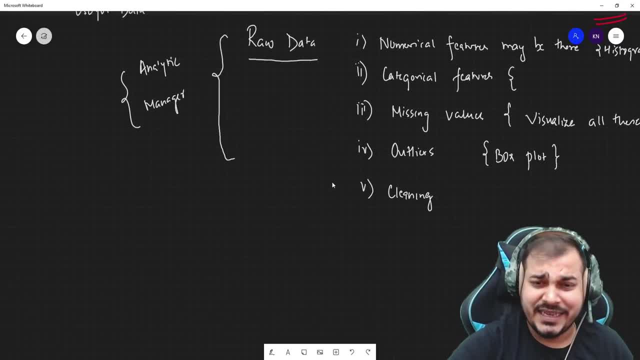 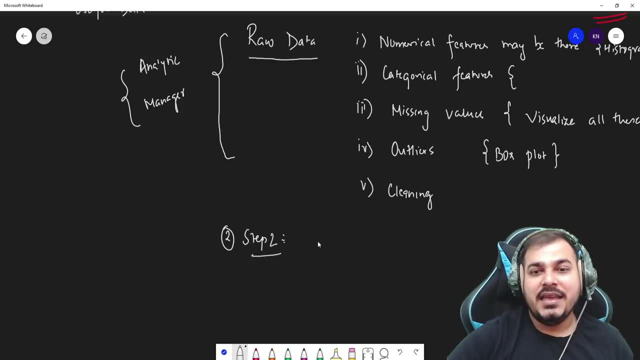 see all these things right now. let's come to the second step. very, very simple now. in the second step, what I always do is that I start handling the missing values. I start handling the missing values very, very important. there are various ways of handling the mean missing values. you may be saying okay. 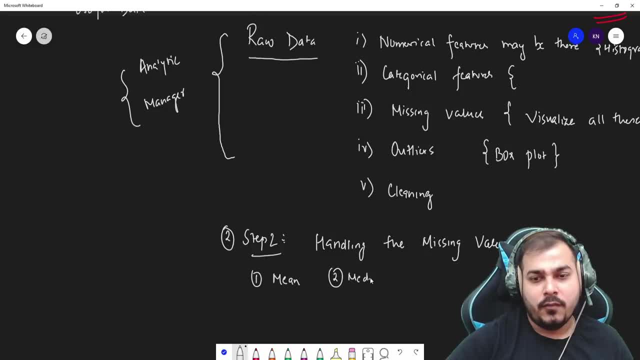 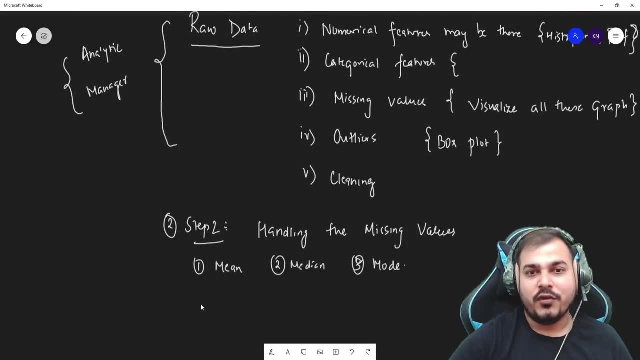 Krish, we may use mean median more. right, all these things right, not only this guy's, not only mean medium more. I'll try to analyze those features. I'll try to see whether there is an outlier in that particular feature. this three, just one, some of the three steps, and we 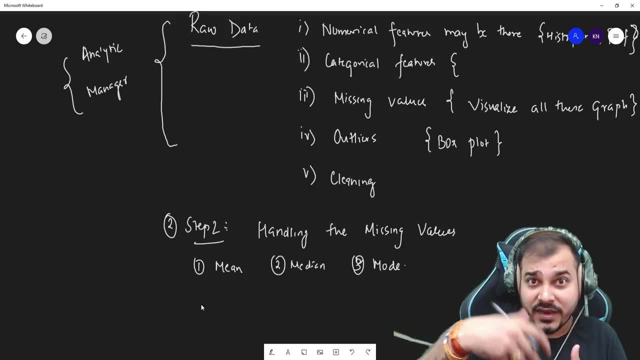 have a lot of various modes, a lot of various ways to handle the missing values. right mean median mode are one of them. you know I may replace some of the features by considering some different, different techniques also, and the entire details is mentioned in my feature engineering playlist again feature. 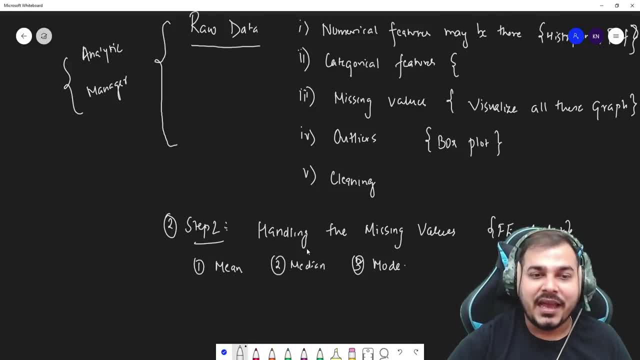 engineering playlist. you know I may analyze it. I may. I may create a lot of box plots to see. okay, if I'm utilizing IQ, are in removing- you know, if you remember there is an formula with respect to IQ- are also to remove the outliers. and after handling the outliers, what I'll do? I'll try to handle the. 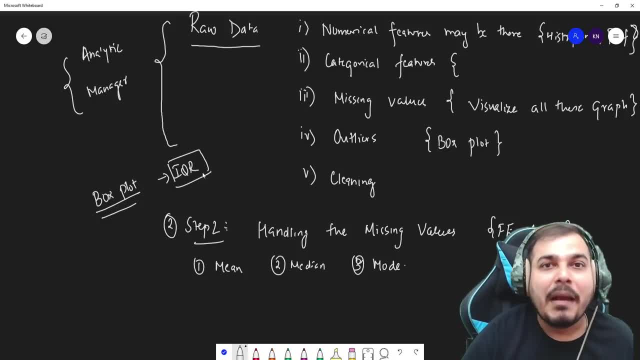 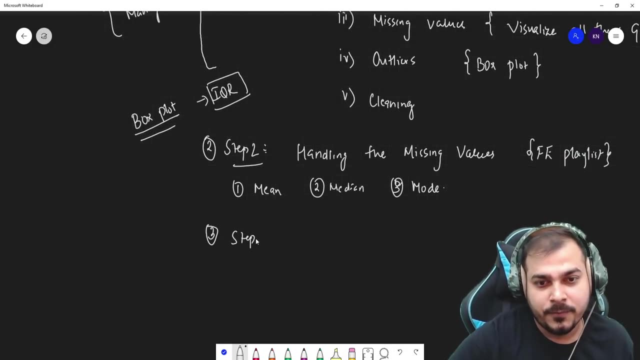 missing values by median. in short, if you don't want the impact of the outlines, you can directly use median or mode. right? so this is basically about the second step, the third step. what I do is that you know step, step three. so in the step three, what I can actually do is that handling. 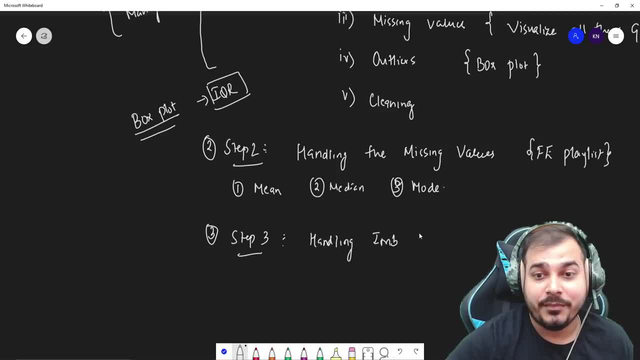 outliers: right, you can handle the outlines. okay, what I can do is, because of you know that I got this, these values- that you can handle outliers, absolutely, you can handle outliers, but there are other options that are available, right, okay. so the third one is involving the outliers. right, the outliers is a very 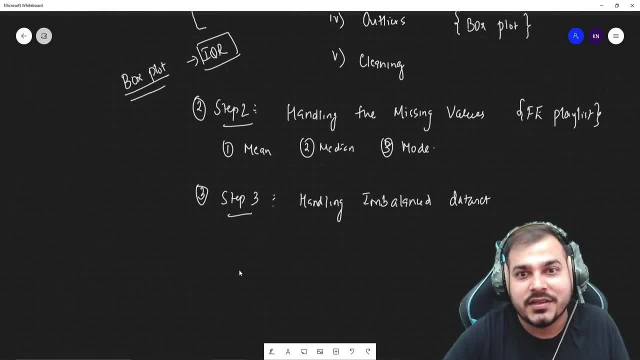 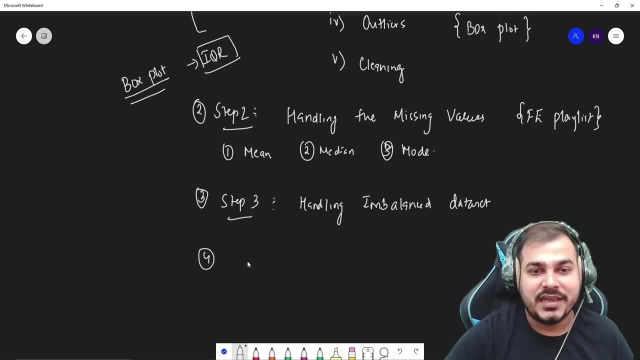 important step. okay, you may get the very bad accuracy and you may be thinking that, okay, you have got an amazing accuracy, but because of the imbalance data, so you may get a very bad one right now. the fourth one that I would like to do is that treating the outliers right. this is also very much important step. 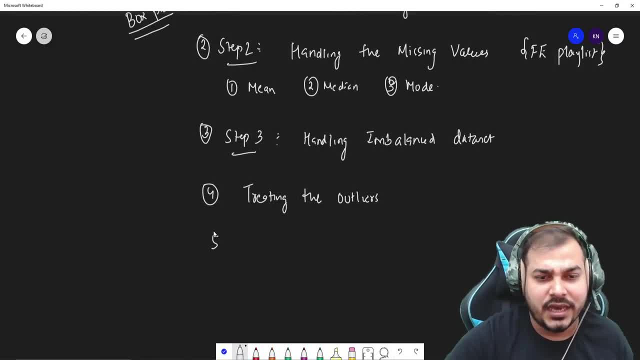 okay, also, which you should definitely explore. i'm just telling you step by step. whatever i do, i'll basically use this and before all the uh, one more step that i can actually do is scaling the data right. scaling the data in the same scale. we use different, different process, like standardization. 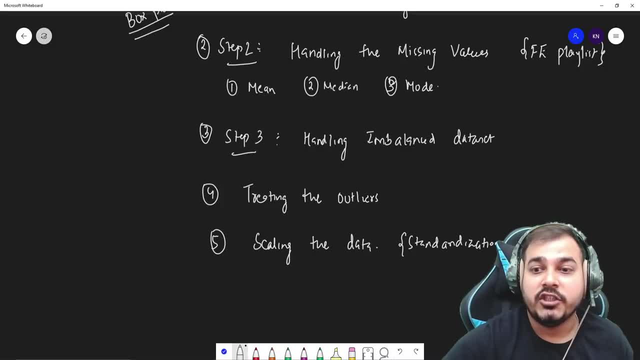 right. standardization, normalization, right, all these techniques we actually used in feature engineering. right coming to the sixth step, uh, this is very, very much important. that is, converting your categorical features, converting the categorical features, categorical features- into numerical features. right, this is the most important step: numerical features. one example: 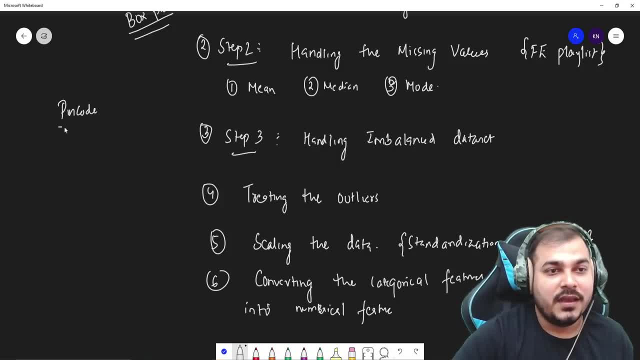 i'll tell you. suppose you have an example like pin code. in pin code you have different, different, different values, right, and here you have the pin code. right and here you have the pin code and here you have the pin code. right and here you have the pin code, right, and here you have so many features. 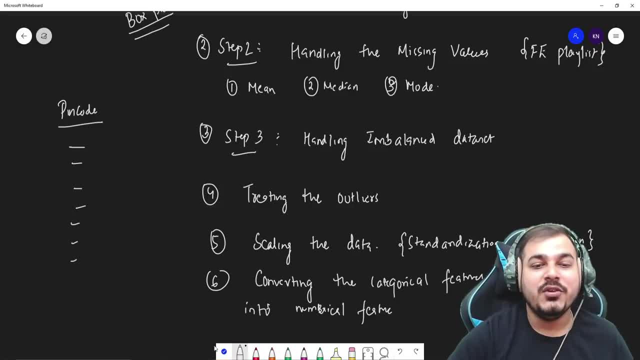 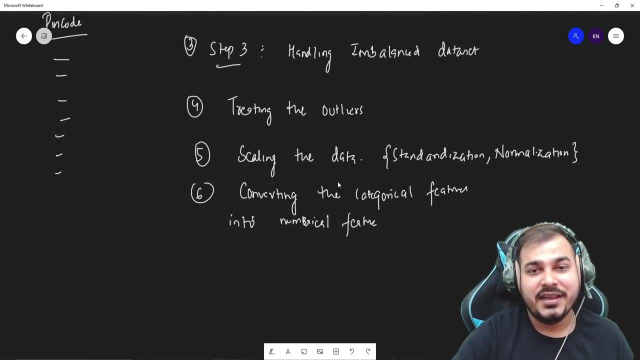 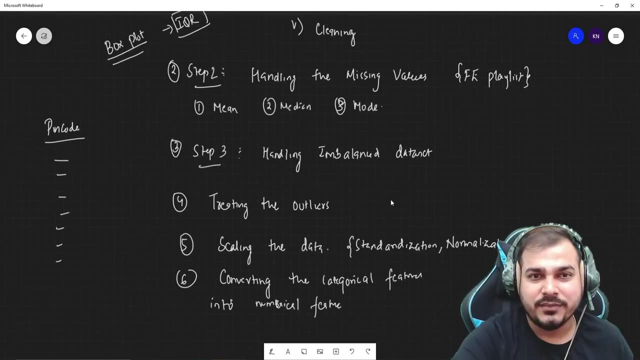 so many unique categories. so what technique you may probably use in order to convert this categorical features into numerical features, and probably you have to actually use this right now. coming to the next step and see all these things, what, what by by this, all these things, what we are actually doing, see, uh, if i go from step one, eda, step two, handling the missing. 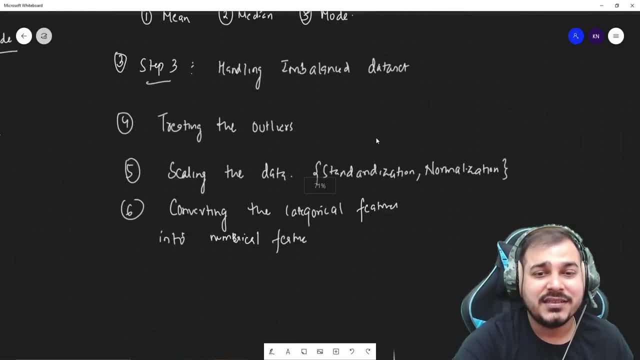 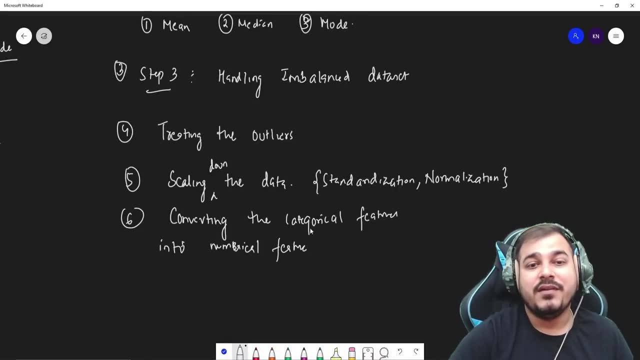 values, handling imbalance data set, treating the outliers, scaling the data, scaling down the data- just write, scaling down the data right, and then converting the category features into numerical features. once I perform all the steps, what I think is that, yes, feature engineering is about 90% completed and don't think that you'll 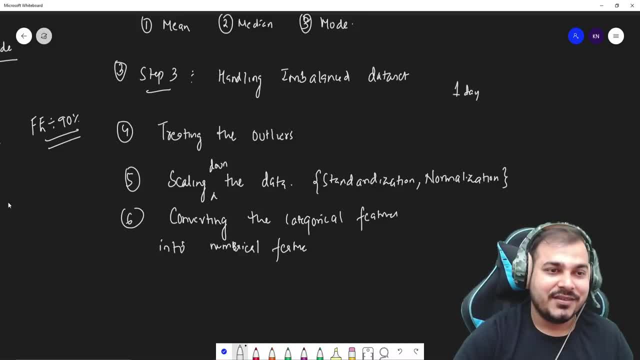 just be able to do it, this in one day or two day. if you have a small data set, obviously I'll say that you will be able to do it in three to four hours. but understand, I have worked with data set where you have 1 million records, right. 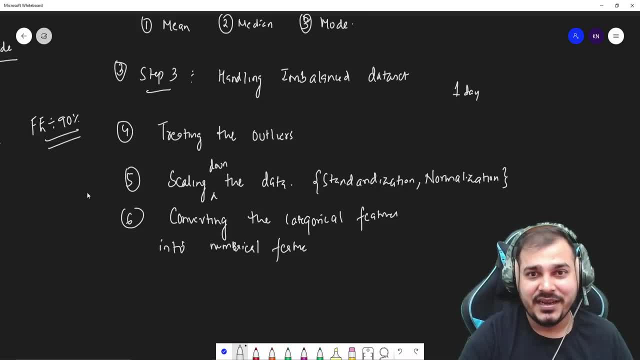 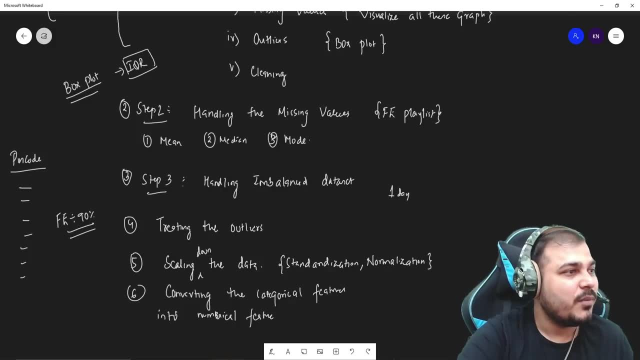 and for doing all these things it takes time, right, always make sure that you follow this process. you always remember these steps, okay? this is very, very much important. let me just check out if I have missed any scaling down category for an outlier treatment. everything is mentioned over here very clearly, okay, so 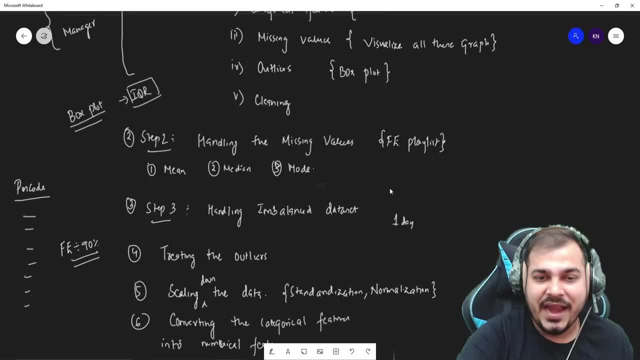 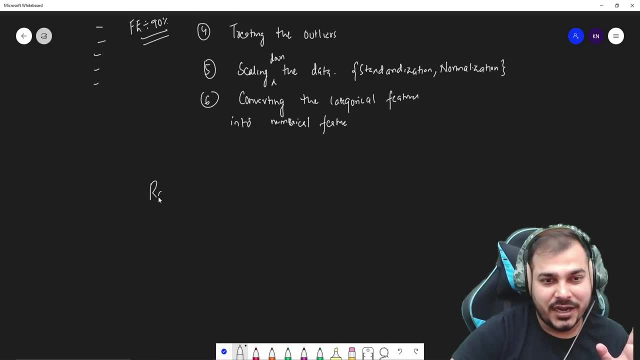 these are most of the steps that we do in the feature engineering and till here, right from here to here. so what has happened? now? see why feature engineering is important. let me talk about it: the raw data, the raw data. in this raw data, you'll have. so 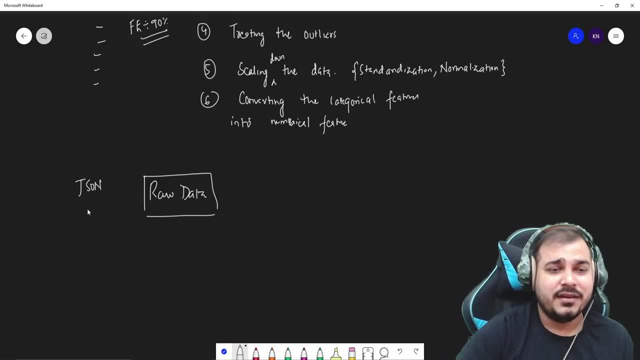 many problems you'll be having. right, it will probably be the JSON format. probably it may be not having proper features. it may be not in the proper format. you know, there may be many things. right: this raw data. after this entire process of feature engineering, you will be having this clean data and this clean data will now 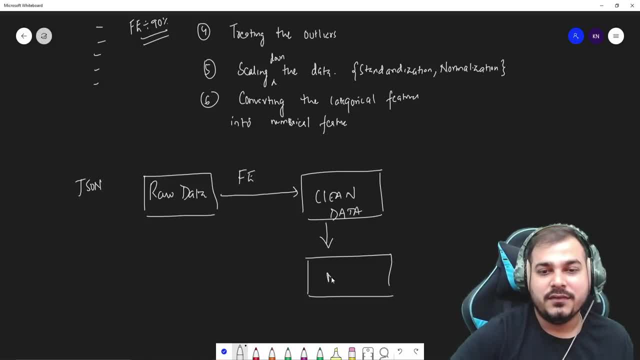 be given to your ML models for the further training purpose. now, when you have the clean data and you are giving your model to for the training purpose, obviously your model is going to give you better results. there is one more step after feature engineering, which is called as feature selection feature. 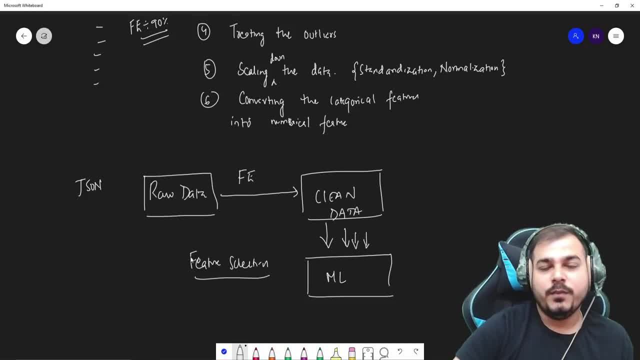 selection is pretty much simple, guys. in feature selection, what we do, we select only those features that are important. now let me tell you that if there are thousand features in your data set, right and out of this entire feature, out of all this thousand features, it is not necessary that all the thousand features 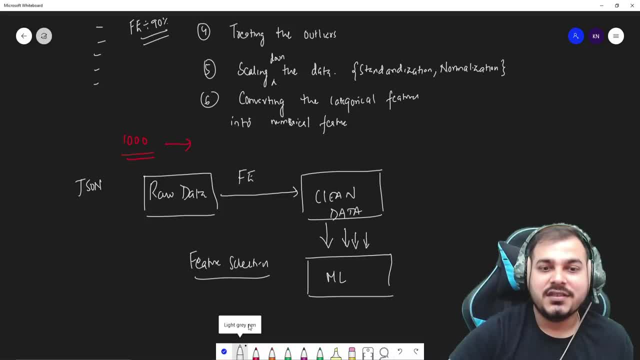 are required. you know, and if you have that many number of features, there is also a term which is called us course of dimensionality. right, and this usually happen when you have many, many features, it is also a curse. so we should take those features that are very important. and in feature selection, what are steps? 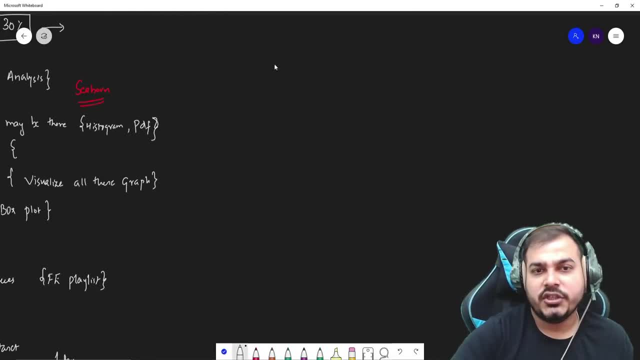 we do- let me write it down over here- in feature selection, what are steps we actually do in feature selection? in feature selection, we perform various steps, right? if you remember right, you have correlation, right, you have one step is basically correlation. and if I talk about more, you also have K neighbors. you can use K neighbors for the feature. 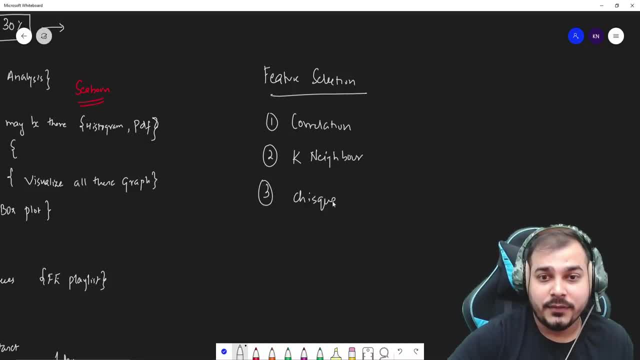 selection purpose. you have chi-square, right, you have chi-square. you have genetic algorithms for doing this, right, genetic algorithms for doing this. you have something called as feature importance- right, these all techniques are there. feature importance, internally uses, extract, reclassify- yet specifically, you use something called as extract, reclassify, right, all these steps, and I 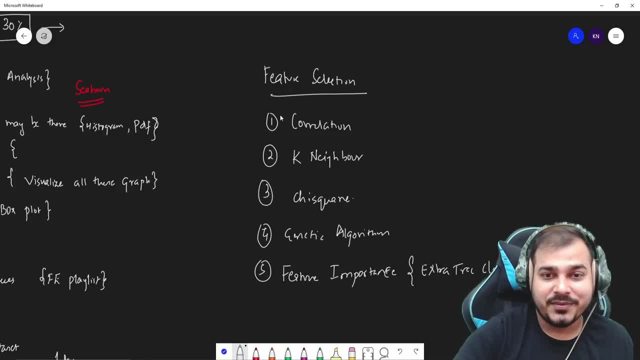 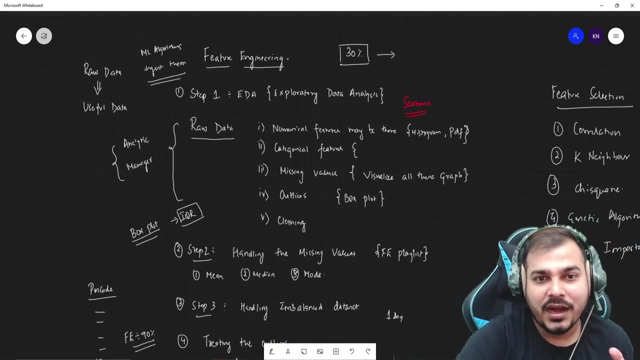 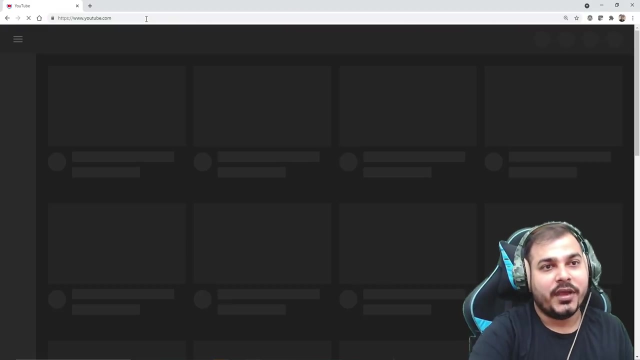 have uploaded videos on this whole right. so all these steps is basically used for selecting. selecting the best features, right, selecting the best features, features. okay, now see, this is the most important step and again, if you are having any confusion with respect to anything, what i'll do is that just just open the youtube channel. okay, go to. 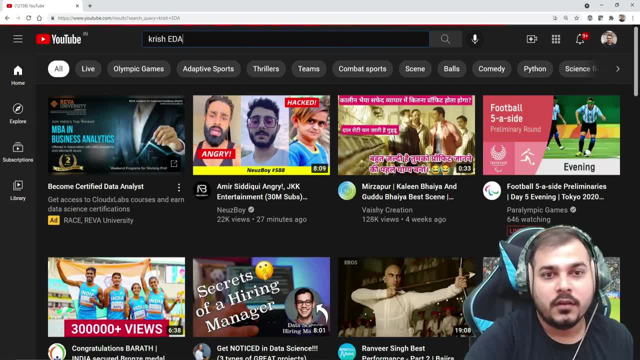 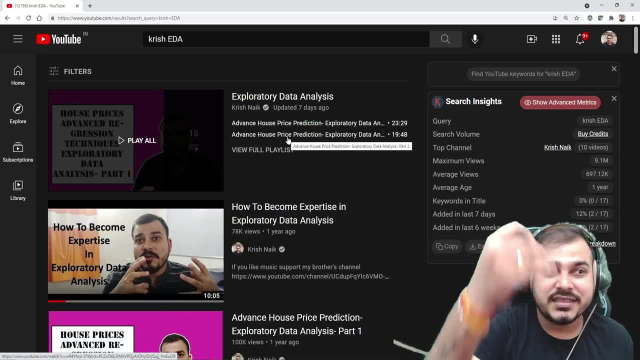 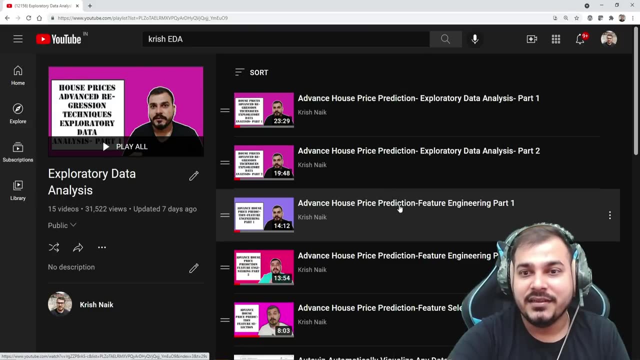 this two playlist. one is krish: eda. okay, so here is your exploratory data analysis playlist. you can go and have a look onto this here in the same steps. i have explained everything. if you go and check out this entire playlist right in the same step: eda, then feature engineering, then feature. 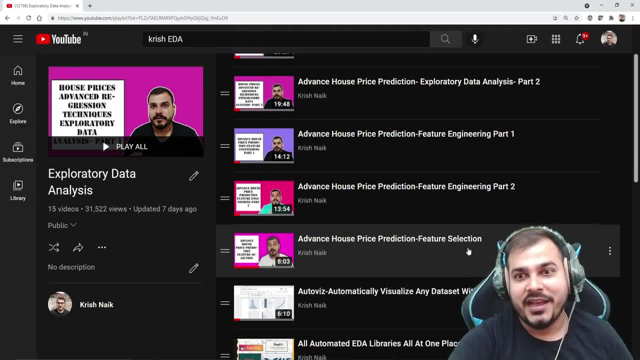 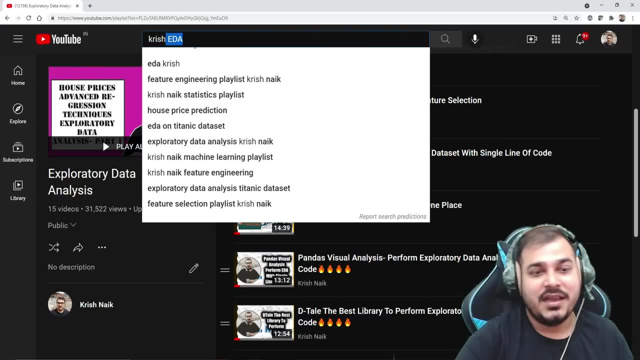 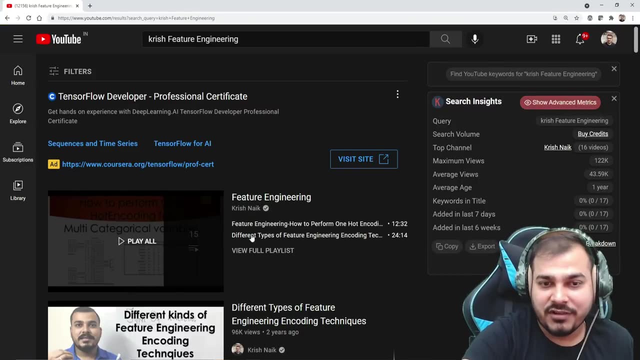 selection in the same step. i've actually explained everything, and here i've also explained the automated eda part. okay, so it will be very much easy. this is the one playlist, and the other playlist is basically about the feature engineering. so this too is must trust me, because 30 percentage. 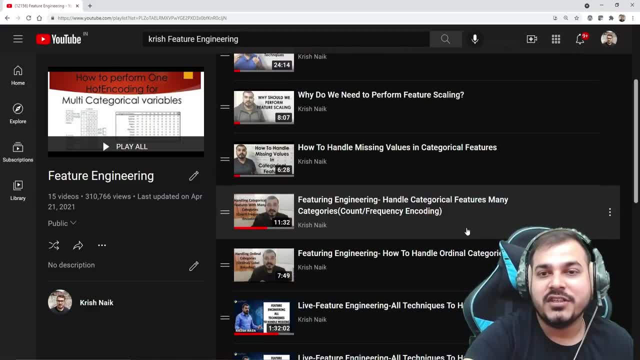 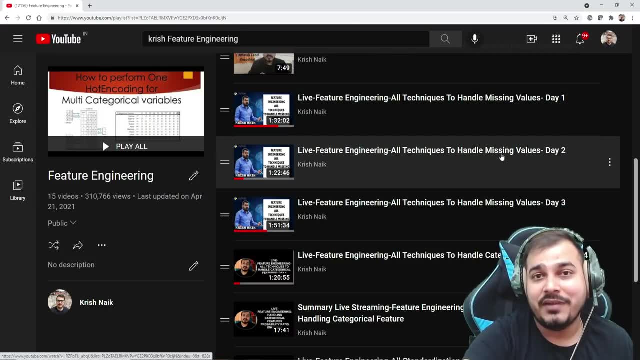 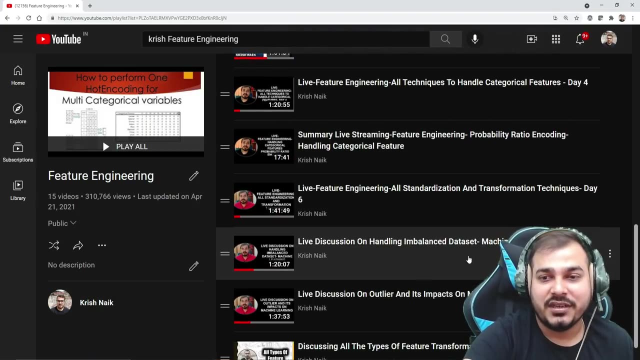 of the time and here all the other different, different types of feature engineering. how do we handle it? category features: how do we handle missing values? see three days, four days on handling missing values. only has been explained. you know how to handle category features. everything is being explained. what is standardization transformation? everything is explained in this. handling missing.